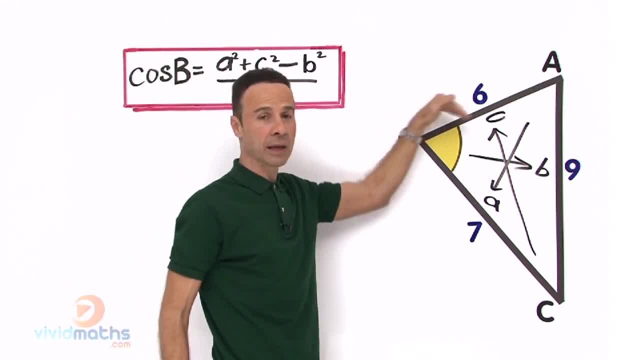 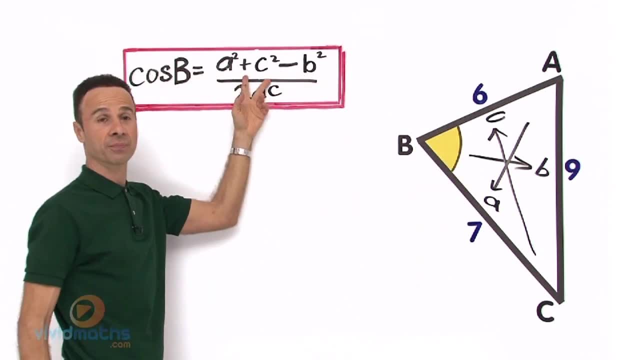 now, what does that mean? It means that the two lengths that are between and cozy with the angle are the two lengths A and C, right here? So you will notice, next to capital B, which is the angle, we have C and A. we have C and A and the opposite length, right here. 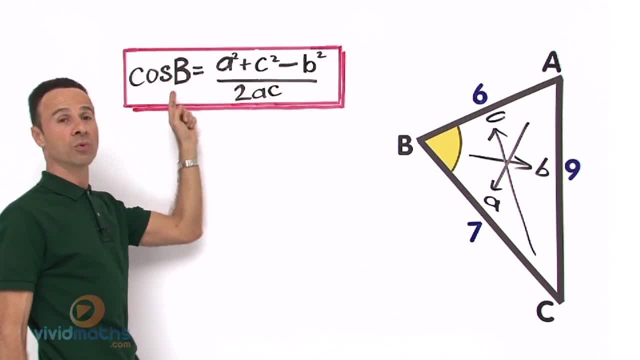 the B is equivalent to the angle we are looking for right on the other side where we subtract. so there is that B right there and it is usually the opposite, and we subtract that in the formula. So let us take these guys and put them in the formula now. yeah, so we have cos B, which 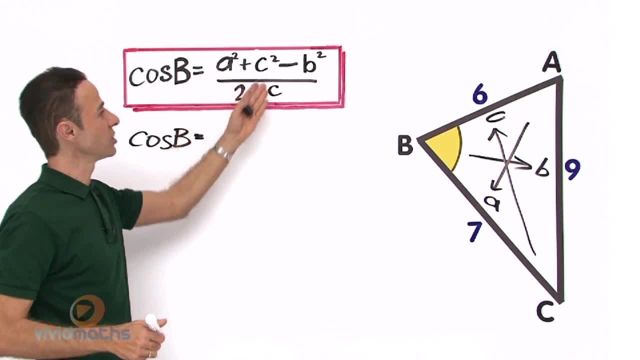 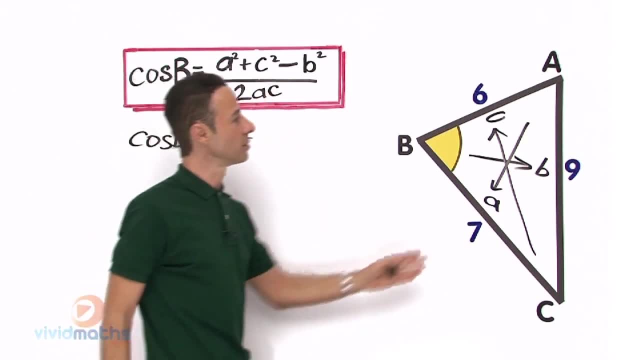 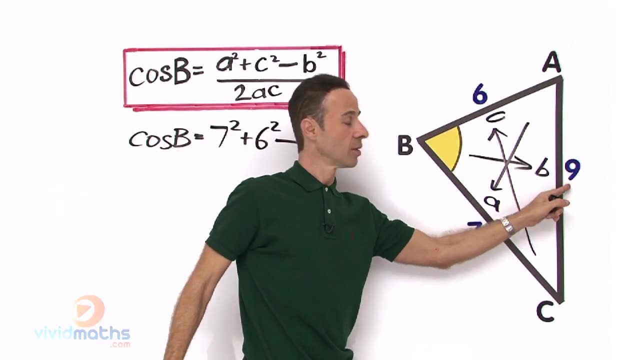 is what we are looking for, and we have A squared and C squared. what do we have for A squared? We have 7 squared, yeah, plus C squared right up there. that is the 6 minus B squared and the B is across here. right there, we have a 9, that is 9 squared all over 2 times A times. 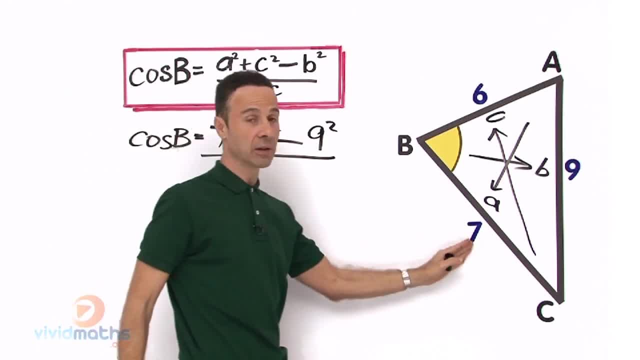 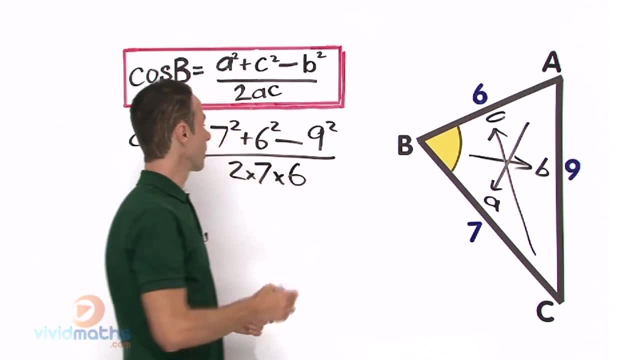 C, which is 2 times, we have A. that is the little A there, right there. 7 times C. if we look at the little C right there, that is 6.. Ok, all we got to do is put that in the formula, Put that into the calculator. so 7 squared plus 6 squared. well, we know that is going. 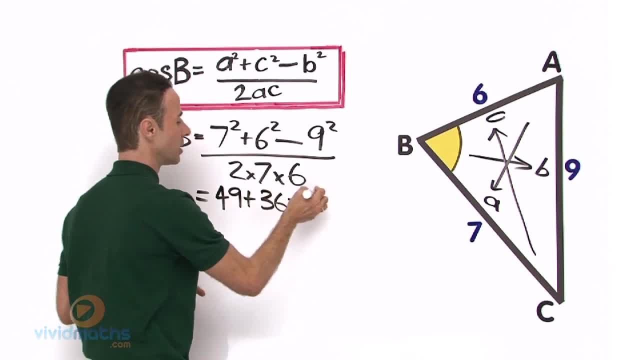 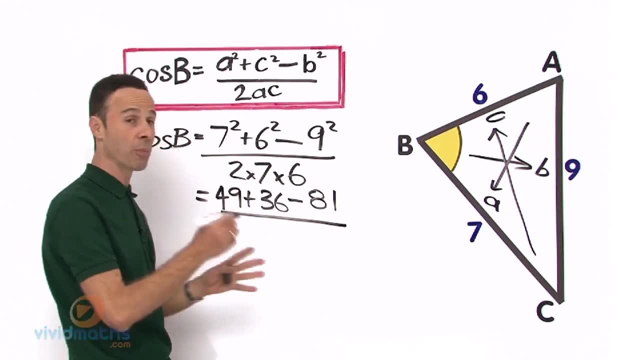 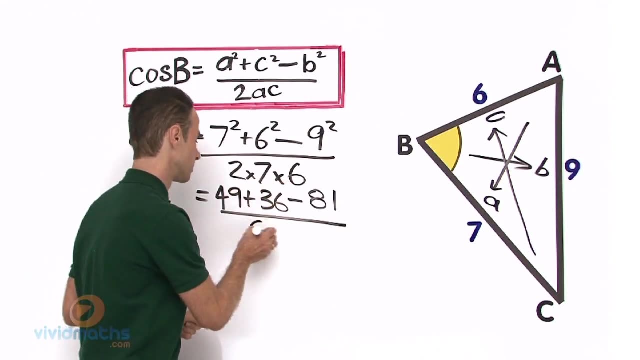 to be 49 plus 36 minus 81. hopefully we will have a small number on the top and a bigger number on the bottom, because we want to get a decimal, that is a zero point or something. 2 times 7 times 6 will give us 84. so that is cos B again. 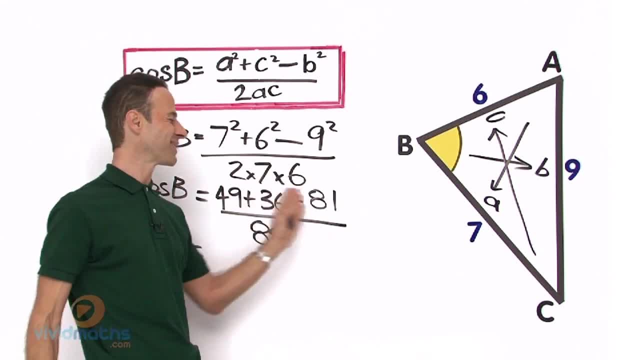 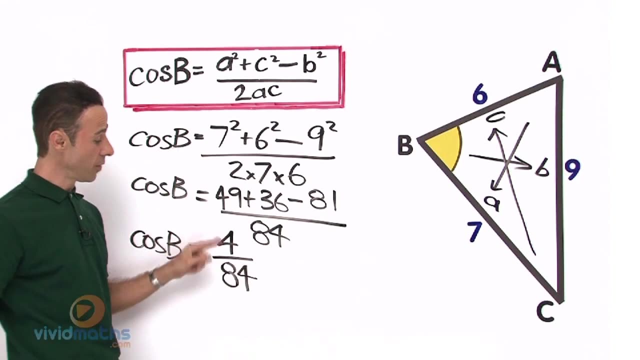 Now that, as we simplify this, 49 plus 36, take away 81 on the calculator will give you a grand total of 4, 4 over 84. so let us do that: 4 divided by 84 will give us a decimal, and that is going to give us: 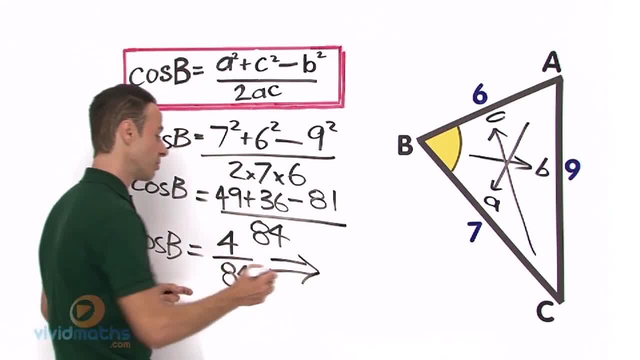 4 divided by 84 is 0.0476.. Ok, So that is what we are going to do. Ok, So that is what we are going to do. Ok, So that is what we are going to do, Ok. 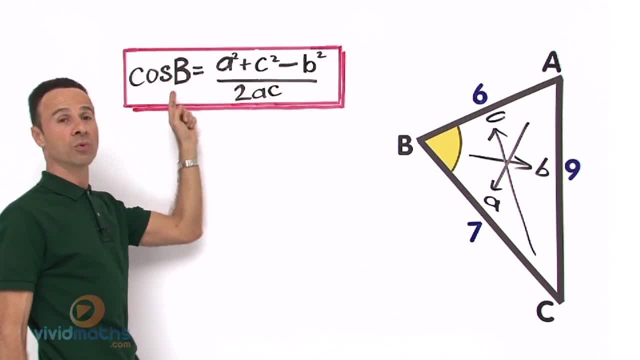 the B is equivalent to the angle we are looking for right on the other side where we subtract. so there is that B right there and it is usually the opposite, and we subtract that in the formula. So let us take these guys and put them in the formula now. yeah, so we have cos B, which 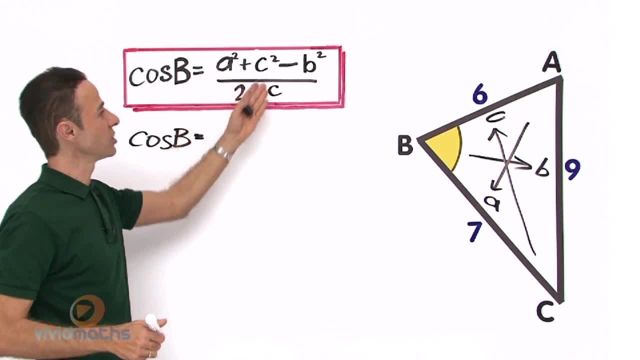 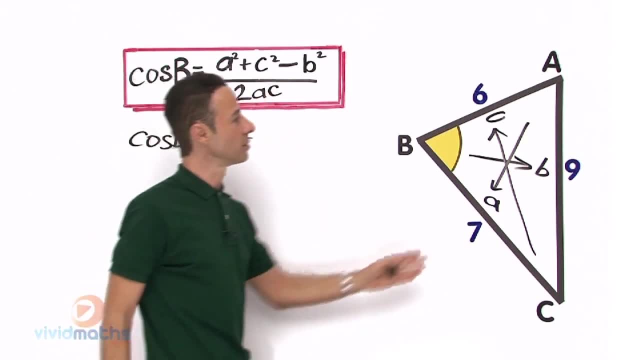 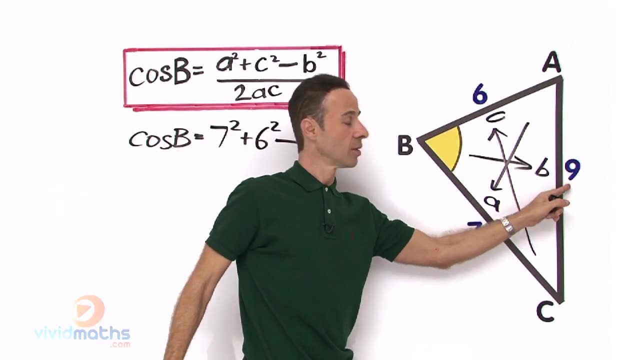 is what we are looking for, and we have A squared and C squared. what do we have for A squared? We have 7 squared, yeah, plus C squared right up there. that is the 6 minus B squared and the B is across here. right there, we have a 9, that is 9 squared all over 2 times A times. 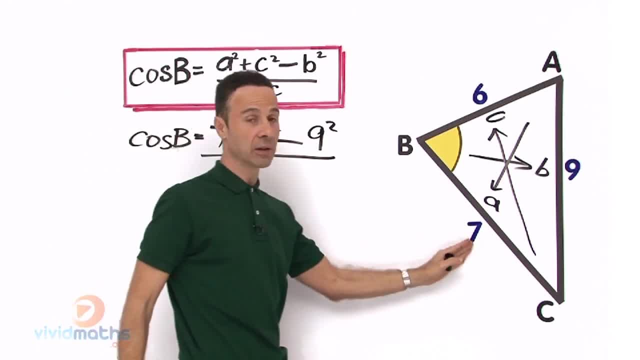 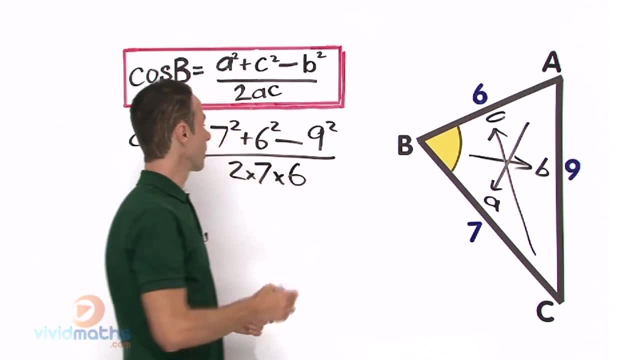 C, which is 2 times, we have A. that is the little A there, right there. 7 times C. if we look at the little C right there, that is 6.. Ok, all we got to do is put that in the formula, Put that into the calculator. so 7 squared plus 6 squared. well, we know that is going. 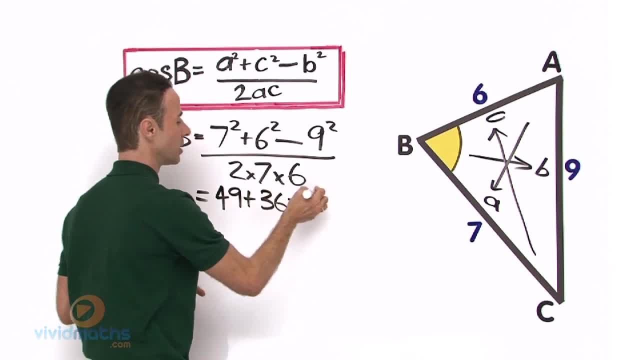 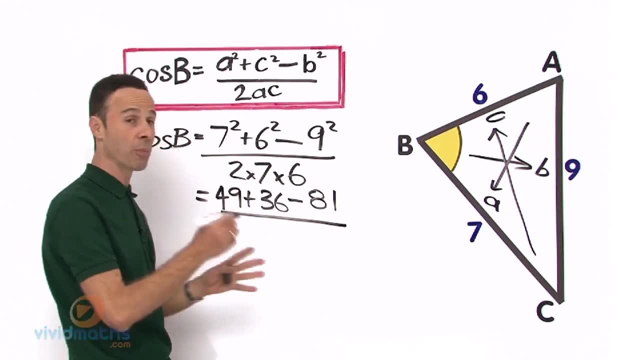 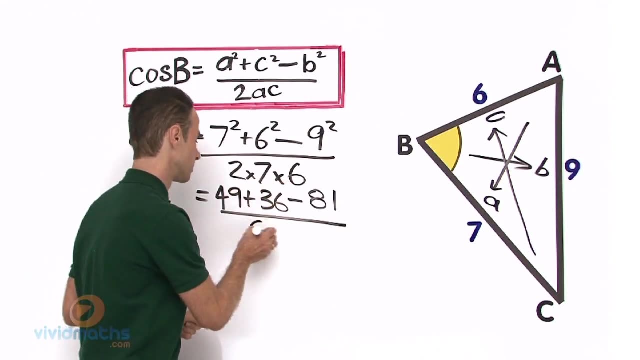 to be 49 plus 36 minus 81. hopefully we will have a small number on the top and a bigger number on the bottom, because we want to get a decimal, that is a zero point or something. 2 times 7 times 6 will give us 84. so that is cos B again. 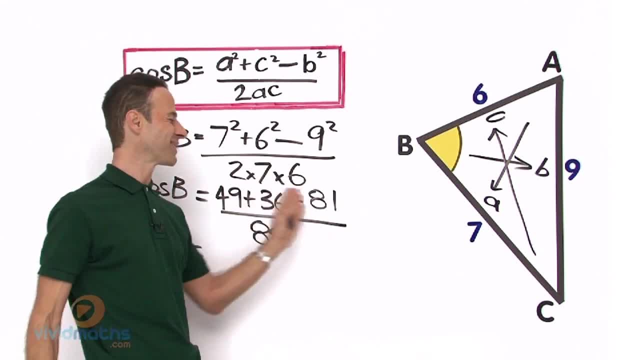 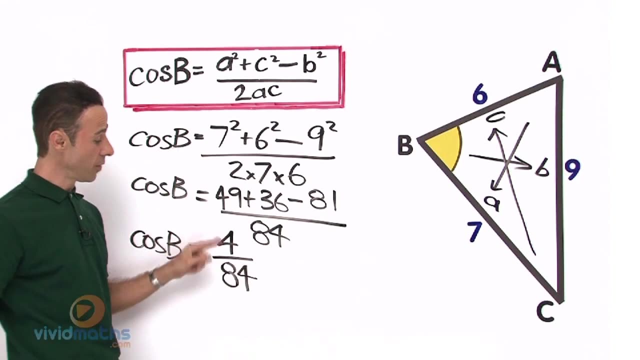 Now that, as we simplify this, 49 plus 36, take away 81 on the calculator will give you a grand total of 4, 4 over 84. so let us do that: 4 divided by 84 will give us a decimal, and that is going to give us: 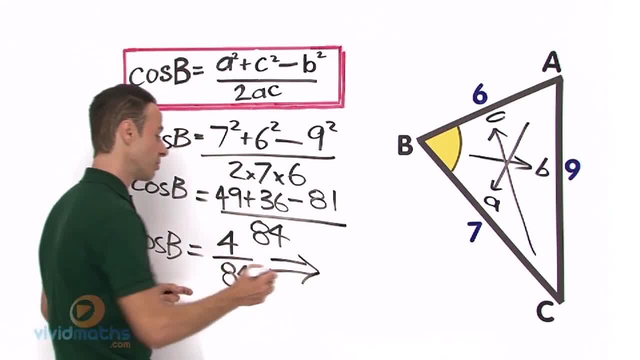 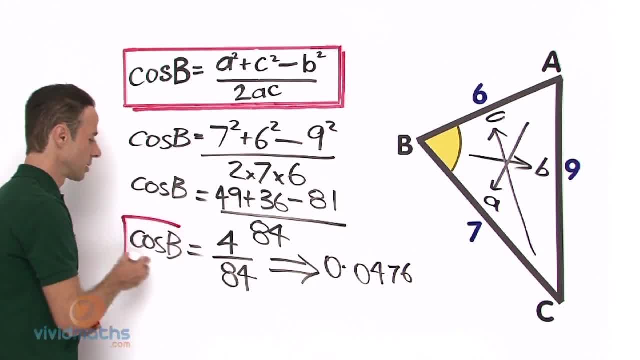 So that is what we are going to do. So that is what we are going to do, Ok. So that is what we are going to do, Ok. Now we are looking for cos B, specifically the B, and it is 0.0476. so let us go to the.